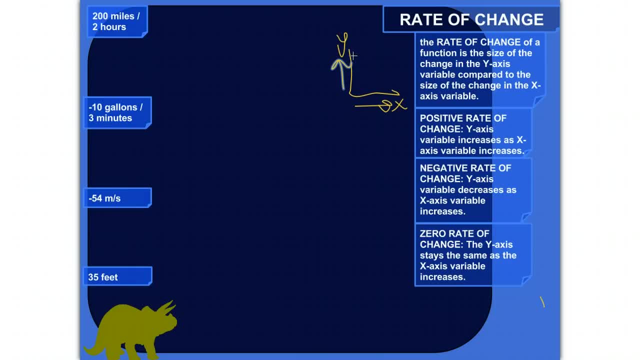 So a positive rate of change be: the y's are going, they're going up when the x's are going up, so it looks like that or that. A negative rate of change is the y variable is decreasing as x increases. So as you go left to right, the y's are dive bombing like that. 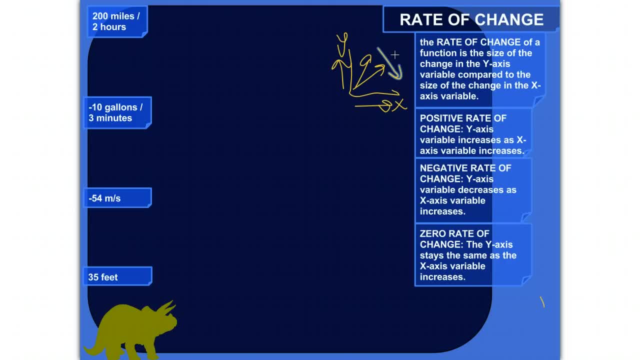 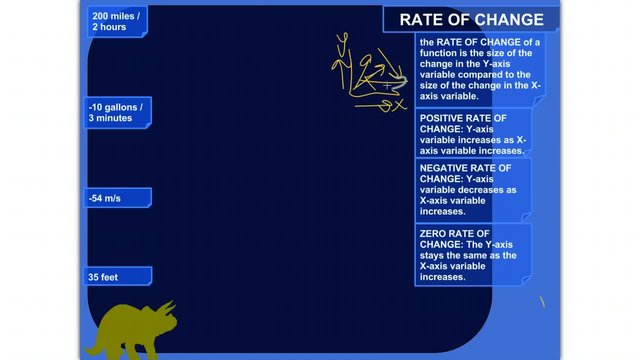 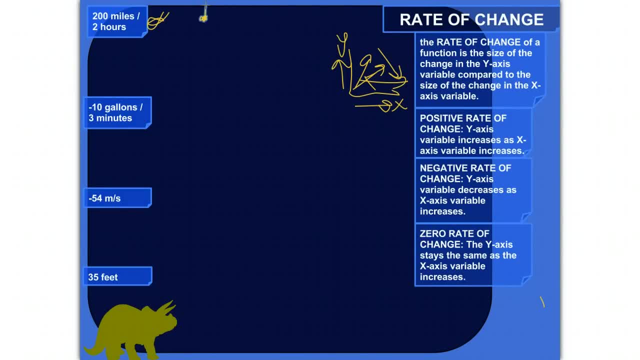 So say like I start here and I'm running very quickly that way And I can measure my distance away from my starting point. And I can measure my distance away from my starting point, You know, every hour. so maybe after one hour I'm 100 miles away, et cetera. 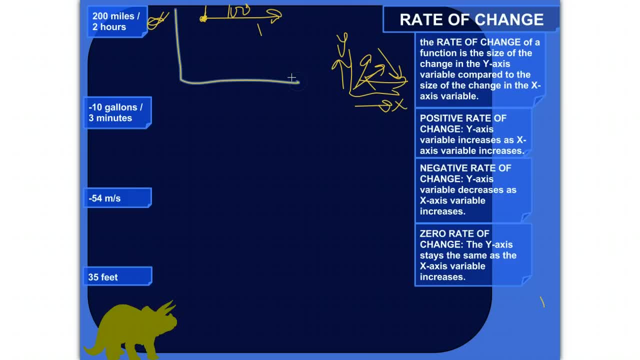 So I could graph this a little coordinate plane here. I'll have time in hours on the x axis and distance in miles on the y axis, And so for every hour, every two hours. excuse me, I'm so if I'm increasing two hours here. 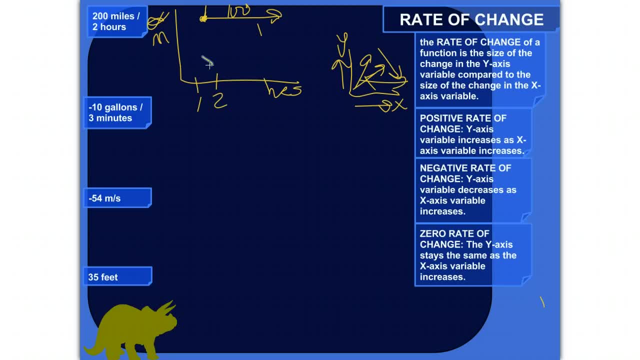 then my y is increasing 200 miles. So here would be a point here. So let's call that 200.. So I'm going up 200 every time I go over 2. And you could reduce that down to 100 miles per one hour or, as we say, 100 miles per hour. 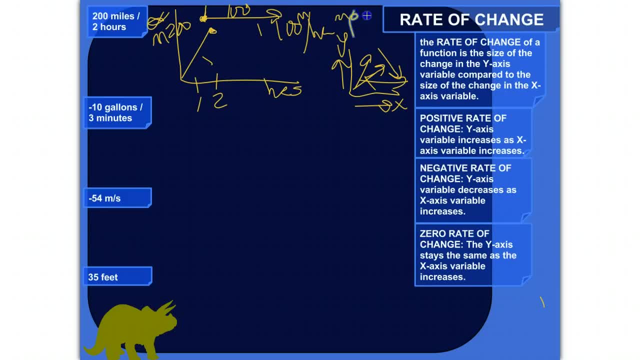 So here's another rate of change here: negative 10 gallons per three minutes. So I'm imagining like a giant tank or something like that with, let's say, water in it. That's real original. And so we've got this big make, kind of like a cone-shaped thing. 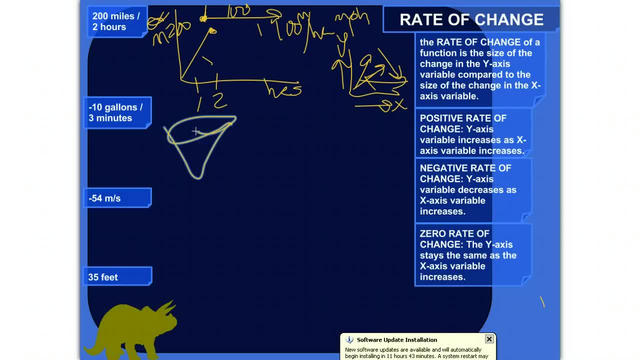 It's got water in it. Let's pretend So. you'll do these in calculus in a few years, Don't worry, It'll be fun. So we're measuring how much water this tank has, And every three minutes it loses 10 gallons. 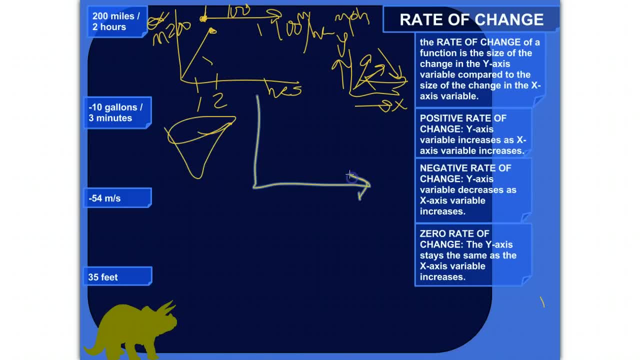 This is a negative rate of change because that y variable is going down. So maybe so if we do minutes on the x axis and gallons on the y axis, maybe it starts out at 100 gallons. So let's say that point is 100.. 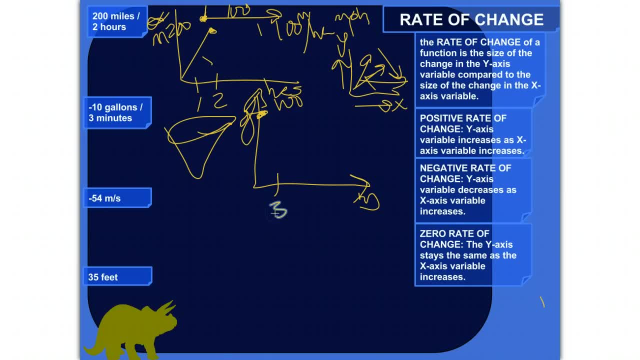 If I've gone three minutes, then it's gone down to 90.. If I go another three minutes to six, it's gone down to 80.. Okay, So you'd see what's called a negative slope. on that I've got another negative rate of change for you. 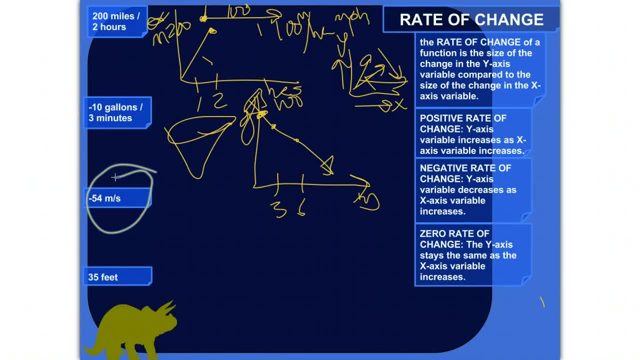 This is negative 54 meters per second, And actually a little side note if you want to impress your friends. that is the terminal velocity of a skydiver, meaning the maximum speed that a skydiver reaches dropping to the earth where the wind resistance actually matches the downward velocity. 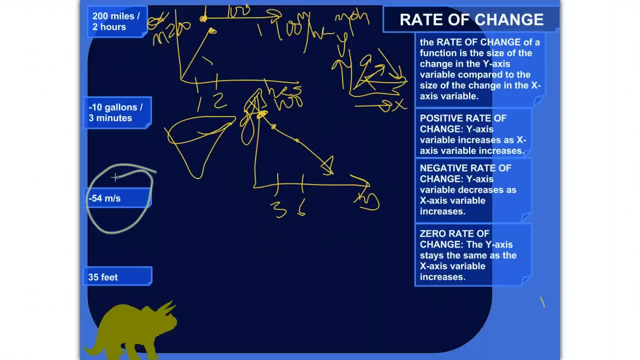 the downward force of gravity. I think it is. I'm not sure if that's quite right. Check out the physics packets and learn some physics, But I think that's right, So let's graph it. So that means I am measuring time in seconds and I'm measuring distance in meters. 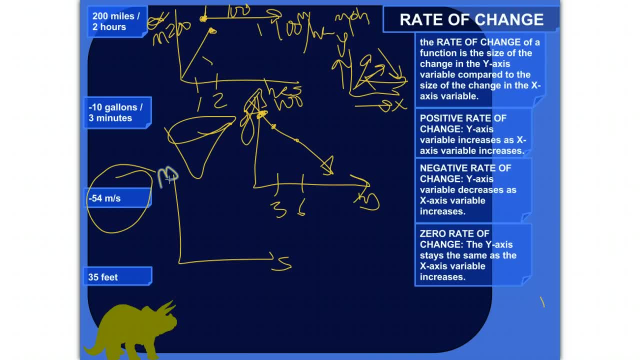 And I am. So if I start up here, every second I'm dropping another 54 meters. So here I've gone down another 54 meters, And here I've gone down another 54 meters. So that would be a negative rate of change. 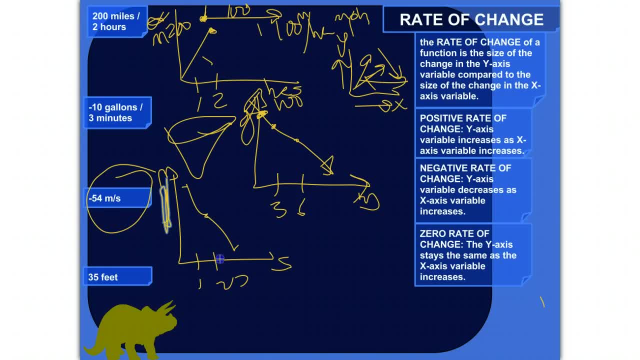 The y-axis variable is decreasing while the x-axis variable is decreasing. So that would be a negative rate of change. The y-axis variable is decreasing while the x-axis variable is decreasing, And then here we have a constant, I imagine. I have no idea why you would ever want to do this, but pretend.